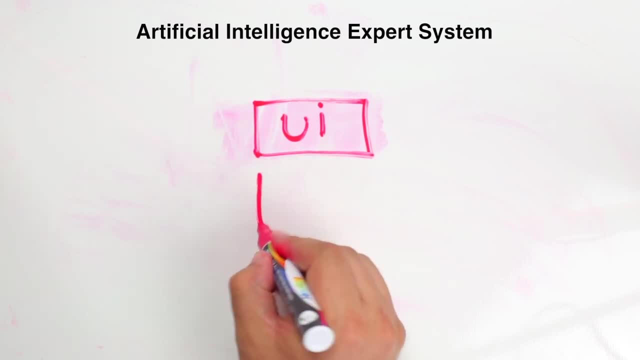 user interface. okay, And then we have another component to the process. It's called an inference interface Engine. And the last component here is the knowledge base. okay, And so let's think of the doctor. here We have a doctor. He has many, many years of experience with diseases detecting. 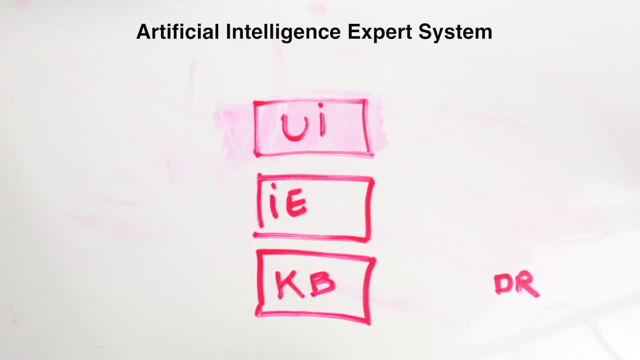 diseases, diagnosing them, knowing what the signs are, And let's input all of that information into the knowledge base. okay, Think of the knowledge base as a database where there's tons and tons of information about how to diagnose diseases. 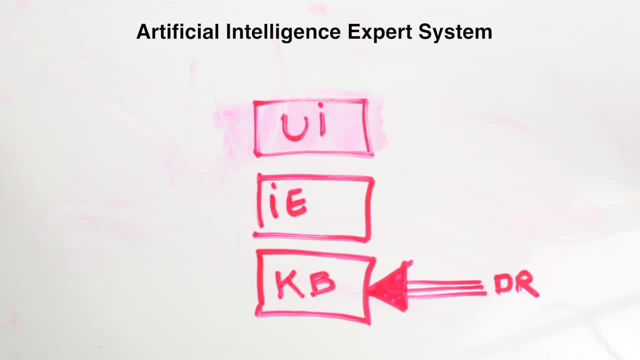 So the knowledge base is essentially a database that contains information, rules about the specific subject, In this case, diseases that are diagnosable by a knowledge base of a doctor. The knowledge base is a collection of objects and their attributes. An object is a result. 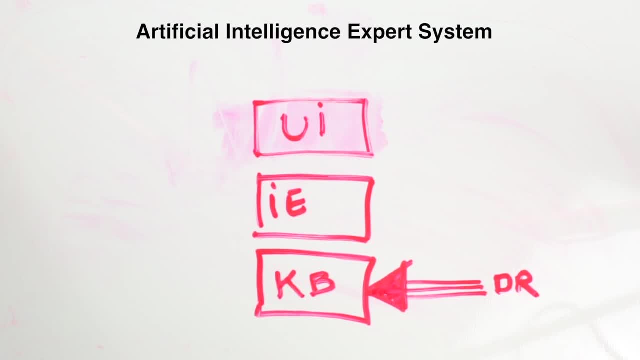 defined by its related rules. Attributes are special rules that help us identify the parameters of the object. The success of any expert system primarily depends on the quality, completeness and accuracy of the information stored in the knowledge base. So if we have erroneous information in the knowledge, 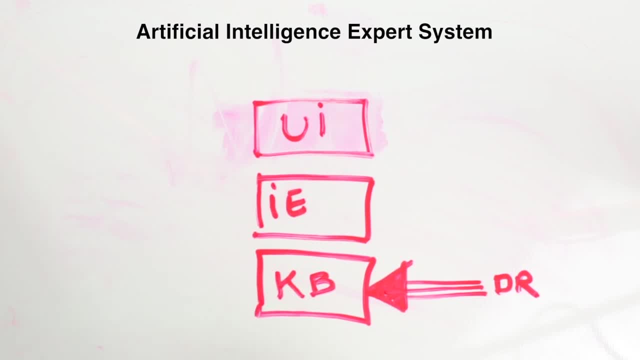 base. whenever we run the expert system, the information that we will receive is not accurate and it's probably not worth anything. So the knowledge base information needs to be really, really high quality. And let's move on to the next part here, and that's the inference engine. The inference engine. 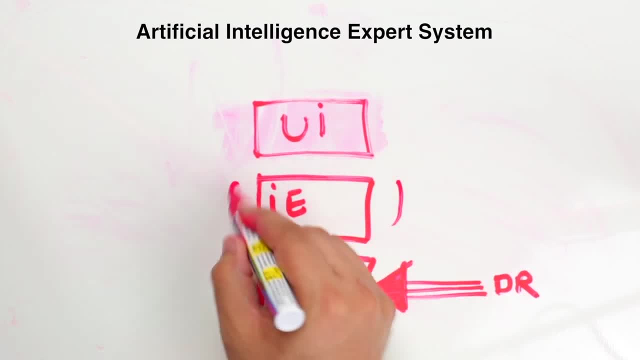 is a primary processing property of the expert system. This, right here, The inference engine uses information in the knowledge base to reach conclusions on different situations. The inference engine attempts to use information collected by the user to find the object that matches So So the user would be the person who actually puts the information here. 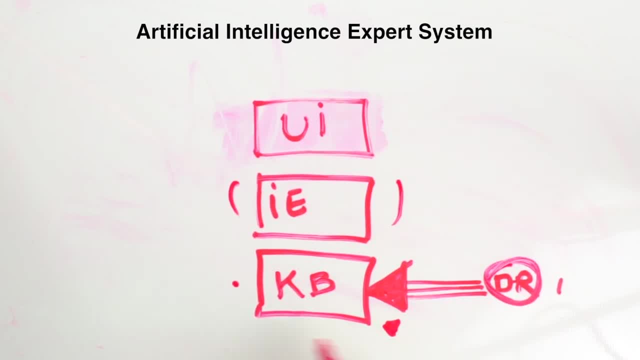 So you know we could have a doctor, but the doctor usually isn't the one putting the information in the knowledge base We usually have like a user. We call it a programmer, developer, engineer, whatever you want to call it. 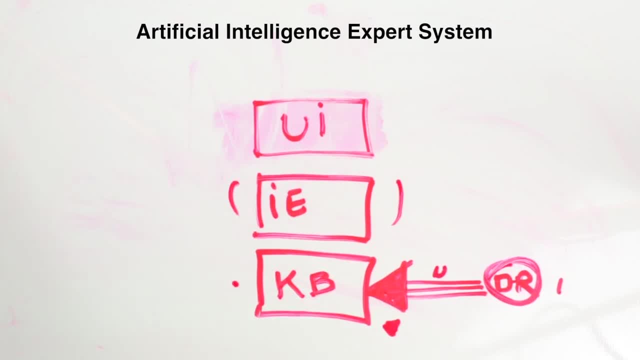 who actually inputs the information in there. Now, there's different types of inference engines. There's a deterministic inference engine. This type of inference engine has an element of certainty. The conclusions drawn are guaranteed to be true. For example, how many protons are found in the nucleus of a hydrogen atom? 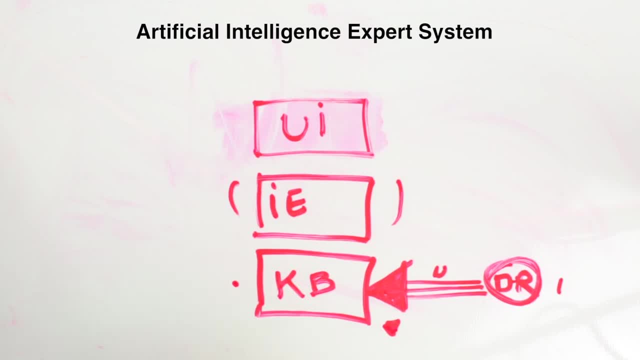 Since this is a known fact, the result is said to be true. And then there's another type of inference engine. It's called a probabilistic inference engine, And this type of inference engine has an element of uncertainty, things that we can't know for sure. 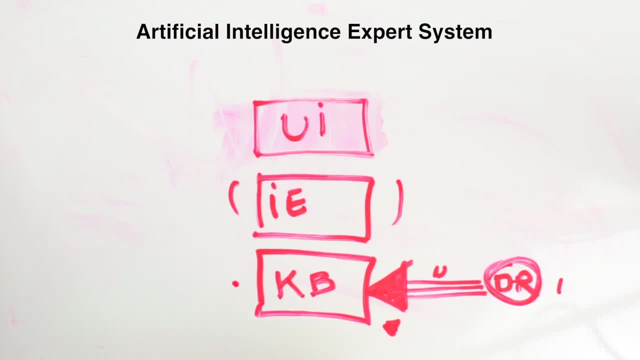 For example, if 100 students take a physics exam, how many of them will pass? It won't give It won't give us a definite answer, but it'll give us an answer. that is probably true. There's different types of inference engine structures. 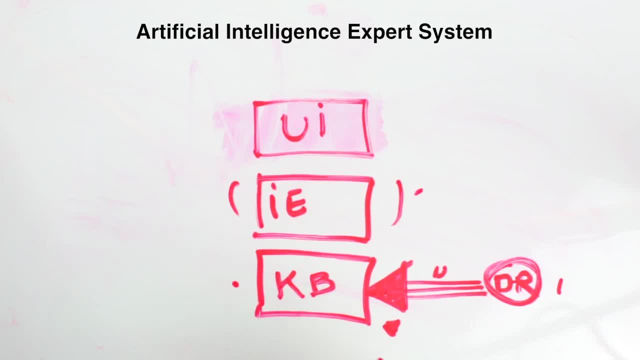 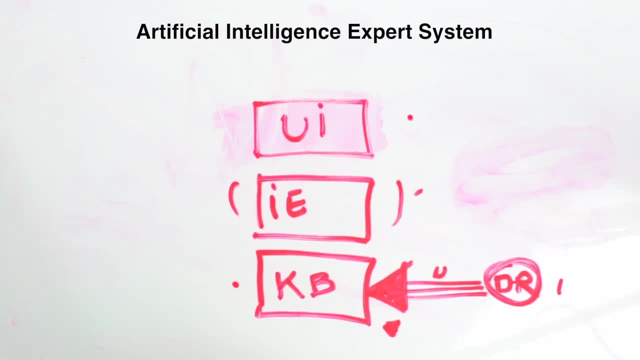 So it has to be used by the user who is well-versed in the task domain. The user of the ES or the expert system need not be necessarily an expert in artificial intelligence to receive the information here. The results should be displayed in the following forms: 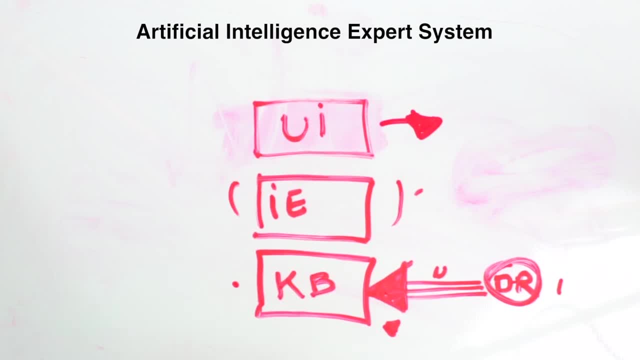 A listing of rule numbers displayed on the screen. verbal narration in natural language or natural language displayed on screen: um. so think of going to the doctor. when you go to the doctor, you present to him um certain symptoms. for example, you might have a cough, okay, and so in this knowledge base, you'll